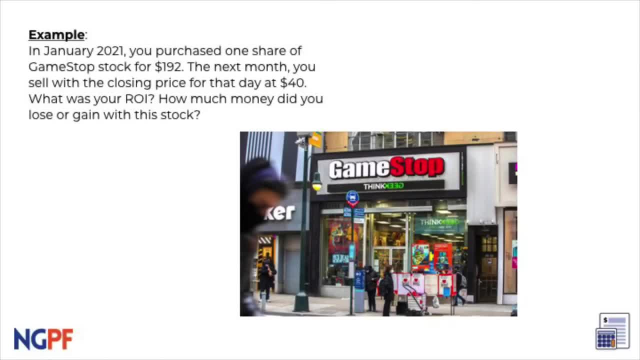 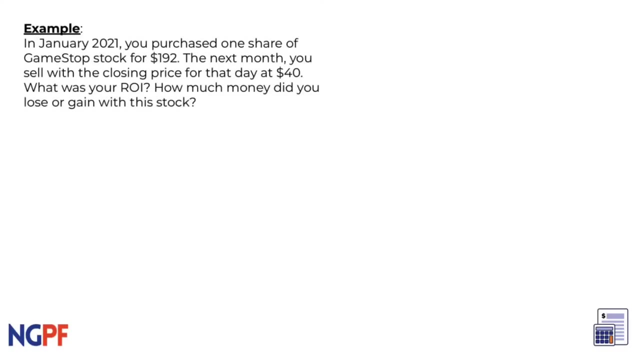 for $192. Then in February you decided you wanted out and sold with one share of GameStop stock for $192.. with a closing price for that day at just $40.. We are asked to calculate our return on investment and how much money we lost or gained with this stock. I'll write the ROI formula here at the top. 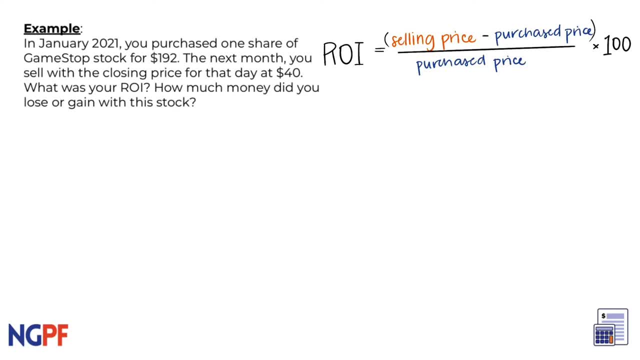 so we can substitute our values. in Looks like we will need our selling price of $40 and our purchase price of $192.. First, we can substitute our given values into the formula. Now that we have our values in the formula, let's evaluate Following order of operations. 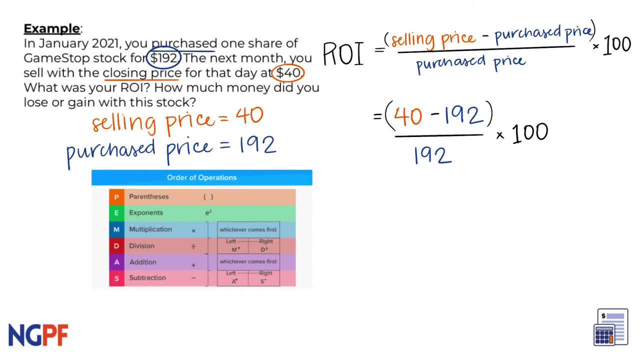 we can carry out what is first in the parentheses. The selling price of $40 minus the purchase price of $192 is equal to negative $152.. We can drop and keep the remainder of the equation, Continuing our order of operations. multiplication and division must be carried out from left to. 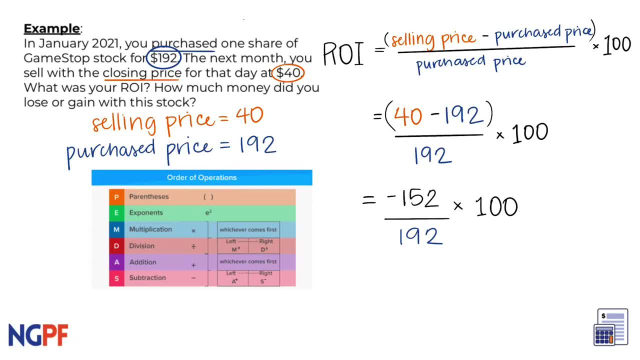 right. So we can take negative $152 and take negative $152.. We can take negative $152 and take negative $152.. We can take negative $152 and take negative $152.. We can take negative $152 and take $152.. We can take negative $152 divided by the purchase price of $192, which gives us negative. 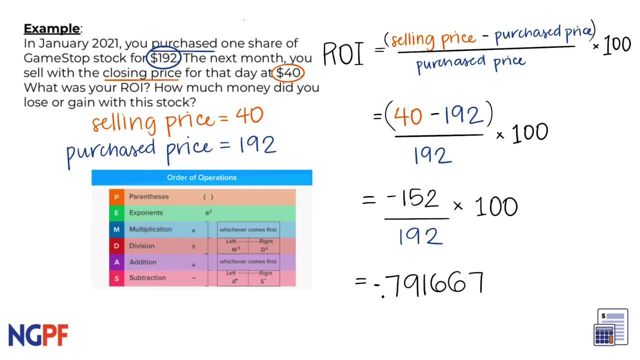 .791667.. The final step is to express the value as a percentage, So we'll multiply by 100, which is giving us our final ROI of about negative 79% Yikes. We typically want our return on investment to be positive and more than the rate of inflation. Looks like this was a rough investment. 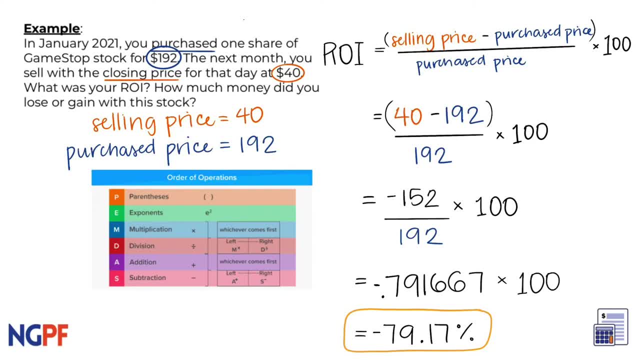 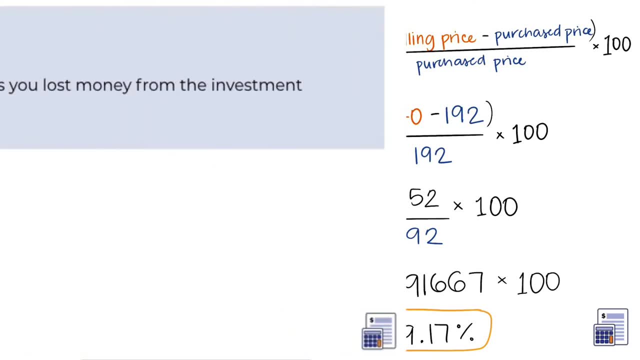 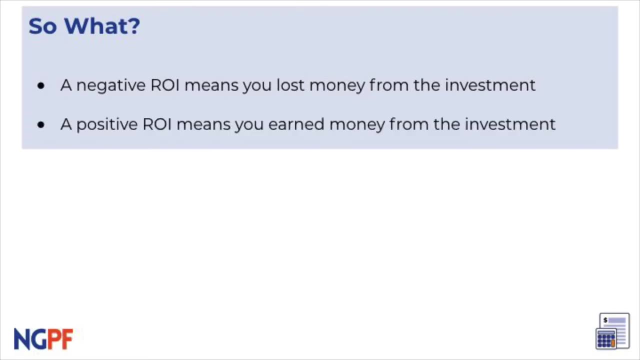 We lost approximately 79% of our initial investment And instead of making money, we lost $152.. So what did we learn from calculating ROI? We see that a negative ROI means we lost money. On the other end, a positive ROI means you earned money from the investment Generally. 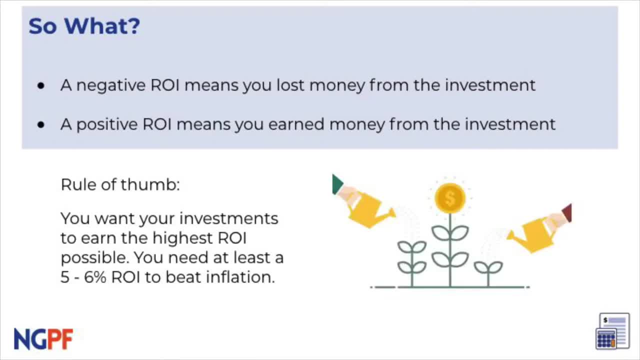 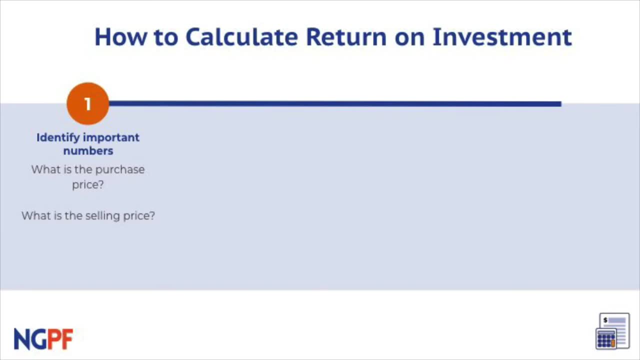 5-6% ROI is a good rule of thumb to beat inflation. Let's review how to calculate ROI. First, identify the selling and purchase price. Then subtract the purchase price from the selling price to find the difference. Next, divide the difference from step 2 by the purchase price.